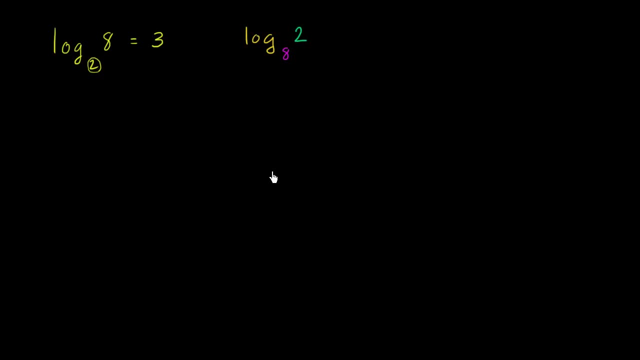 Now this is interesting. I'll give you a few seconds to think about it. Well, we're asking ourselves- or this will evaluate to the exponent- that I have to raise 8 to to get to 2.. So let's think about that in another way. 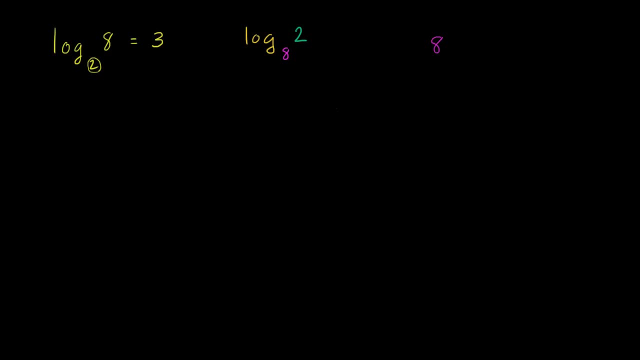 So we could say 8 to some power, and that exponent that I'm raising 8 to is essentially what this logarithm would evaluate to: 8 to some power is going to be equal to 2.. Well, if 2 to the third power is 8,, 8 to the 1. 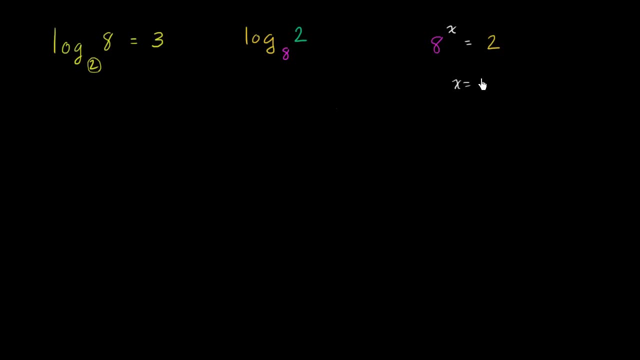 third power is equal to 2.. So x is equal to 1 third. 8 to the 1 third power is equal to 2.. Or you could say: the cube root of 8 is 2.. So in this case x is 1 third. 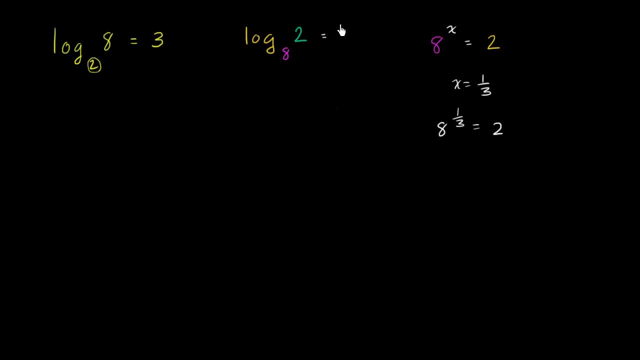 This logarithm right over here will evaluate to 1 third Fascinating. Let's mix it up a little bit more. Let's say we had the log base 2.. Instead of 8, let's put a 1.. Let's put a 1 eighth, right over here. 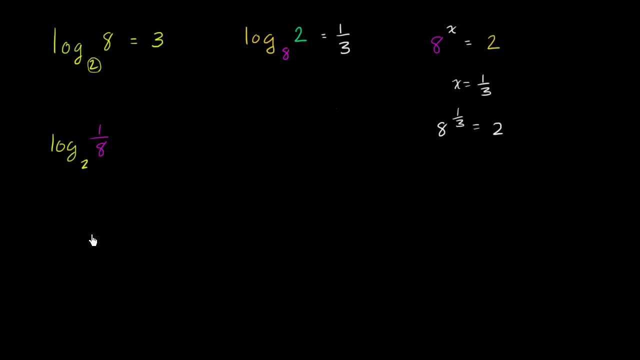 So I'll give you a few seconds to think about that. Well, it's asking us- or this will evaluate to the exponent that I have to raise 2 to to get to 1 eighth. So if we said that this is equal to x, 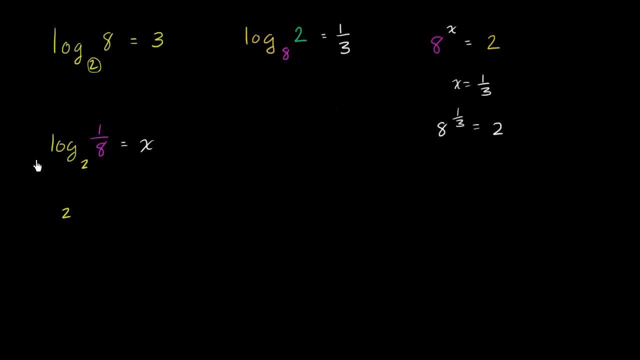 we're essentially saying 2 to the x power is equal to 1 eighth. Well, we know 2 to the third power. Let me write this down. We already know that 2 to the third power is equal to 8.. If we want to get to 1 eighth, which is the reciprocal of 8,, 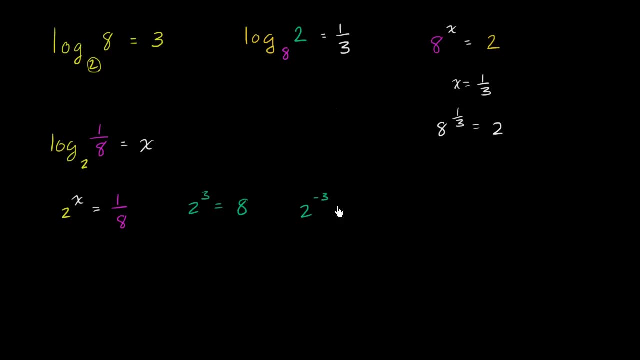 we just have to raise 2 to the negative 3 power, 2 to the negative 3 power is 1 over 2 to the third power, which is the same thing as 1 over 8.. So if we're asking ourselves what exponent 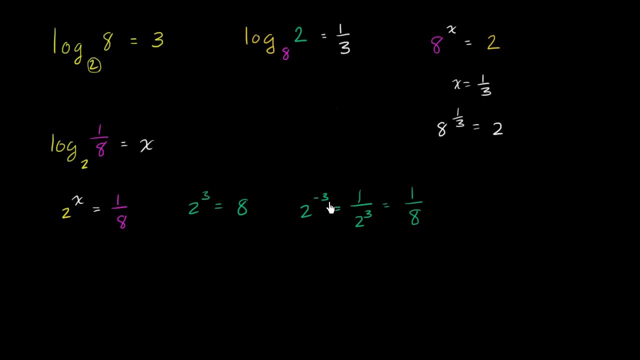 do we have to raise 2 to to get to 1 eighth, Well, we have to raise it to the negative 3 power. So x is equal to negative 3.. This logarithm evaluates to negative 3.. Now, let's really really mix it up. 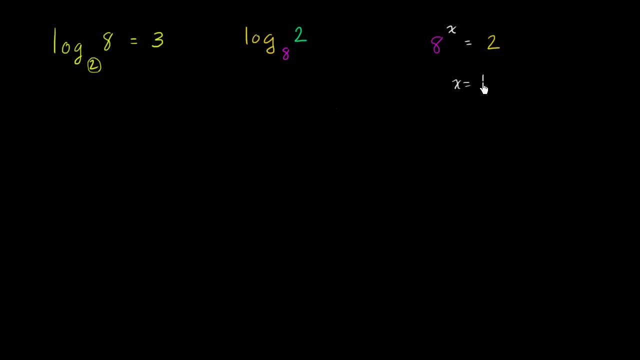 is equal to 2.. So x is equal to 1 third, 8 to the one third. power is equal to 2.. Or you could say: the cube root of 8 is 2.. So in this case x is 1 third. 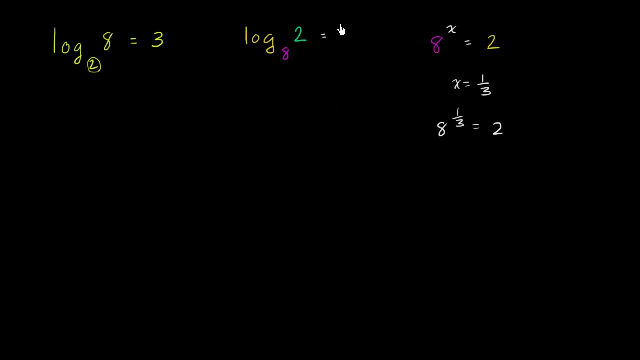 This logarithm right over here will evaluate to 1 third Fascinating. Let's mix it up a little bit more. Let's say we had the log base 2. Instead of 8, let's put a 1. 1 eighth, right over here. 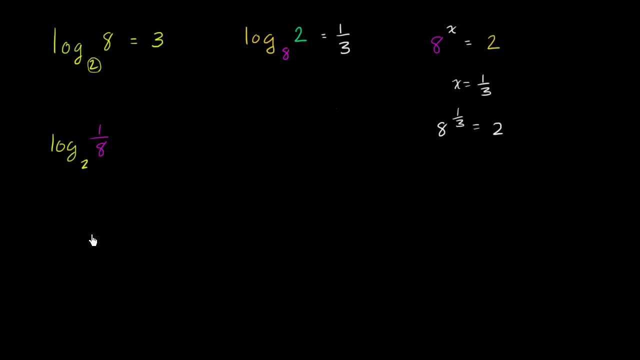 So I'll give you a few seconds to think about that. Well, it's asking us- or this will evaluate to the exponent that I have to raise 2 to to get to 1 eighth. So if we said that this is equal to x, 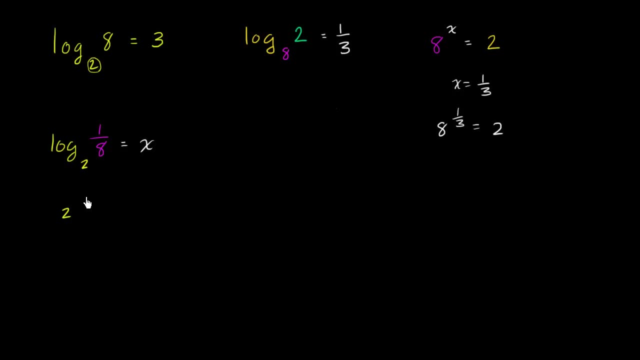 we're essentially saying 2 to the x power is equal to 1 eighth. Well, we know 2 to the third power. Let me write this down. We already know that 2 to the third power is equal to 8.. If we want to get to 1 eighth, which is the reciprocal of 8,, 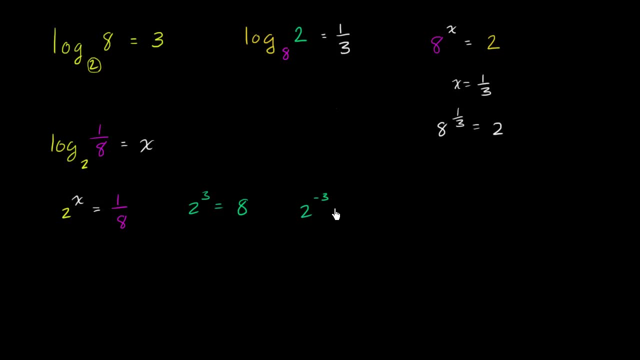 we just have to raise 2 to the negative 3 power, 2 to the negative 3 power is 1 over 2 to the third power, which is the same thing as 1 over 8.. So if we're asking ourselves what exponent 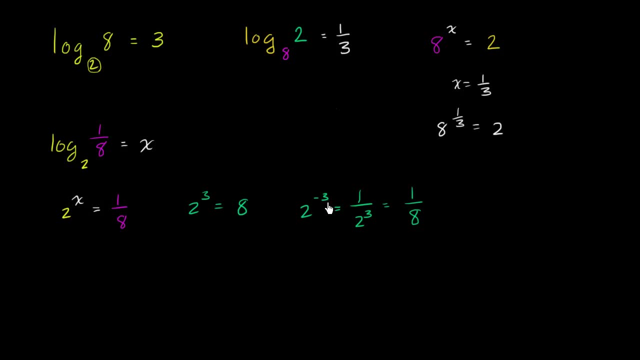 do we have to raise 2 to to get to 1 eighth? Well, we have to raise it to the negative 3 power. So x is equal to negative 3.. This logarithm evaluates to 1 eighth. This logarithm evaluates to negative 3.. 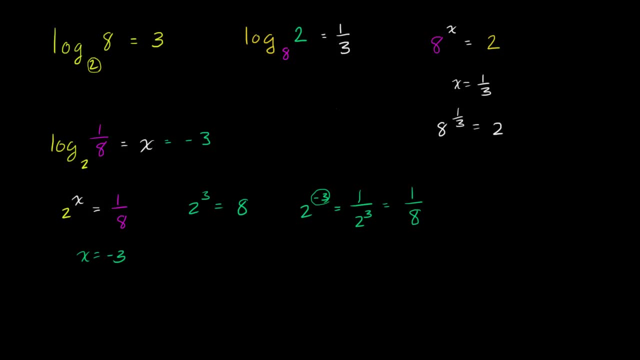 Now let's really really mix it up. What would be the log base 8 of 1, 1 half. What does this evaluate to? Let me clean this up so that we have some space to work with. As always, we're saying what power? 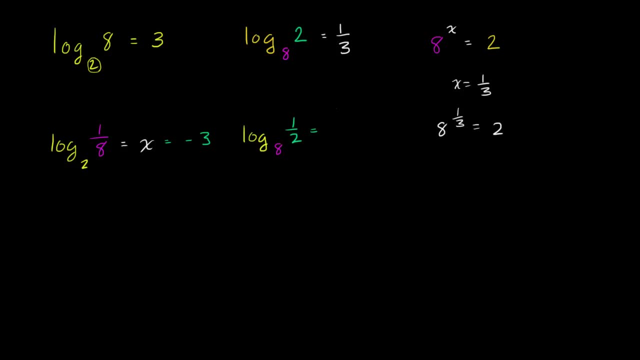 do I have to raise 8 to to get to 1 half. So let's think about that a little bit. We already know that 8 to the 1 third power is equal to 2.. If we want the reciprocal of 2 right over here, 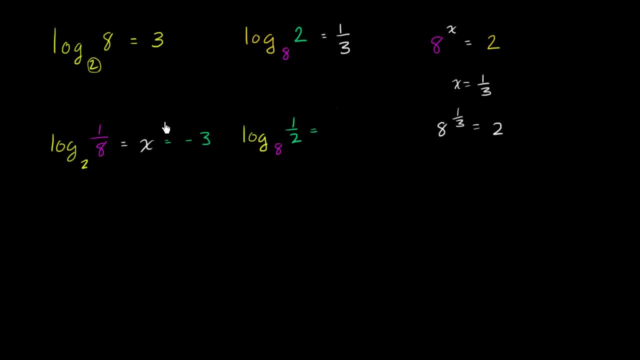 we have to just raise 8 to the negative 1 third. So let me write that down: 8 to the negative 1 third power is going to be equal to 1 over 8 to the 1 third power, And we already know the cube root of 8,. 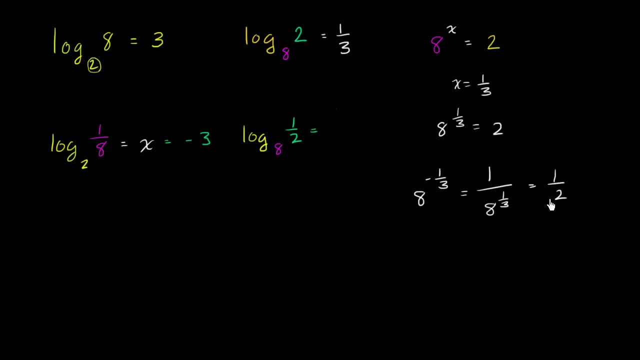 or 8 to the 1 third power is equal to 2.. This is equal to 1 half. So the log base 8 of 1 half is equal to well the power after I raise 8 to 2 to get to 1 half. 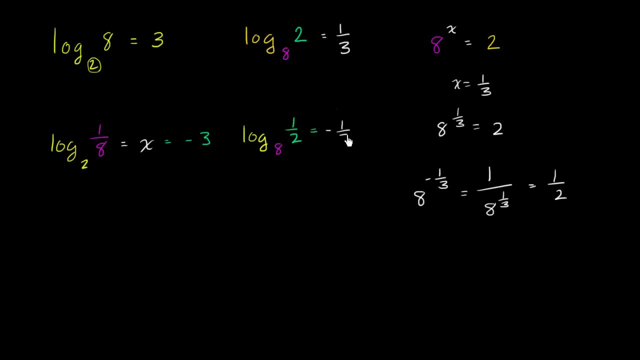 is negative 1 third Equal to negative 1 third. I hope you enjoyed that as much as I did. 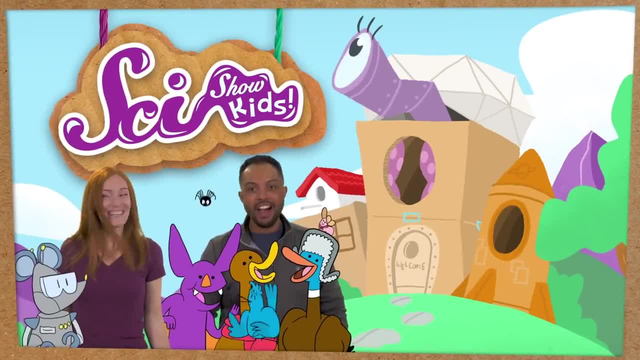 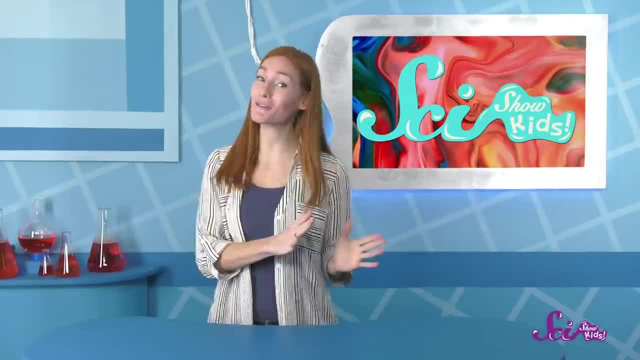 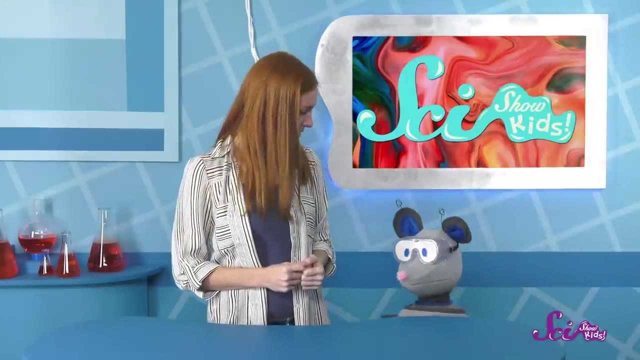 Hi there. We were just about to head over to a nearby hill to draw some of the beautiful flowers that we can see from there. Squeaks went to grab his crayons and he should be back any minute. Oh, what's wrong, Squeaks? 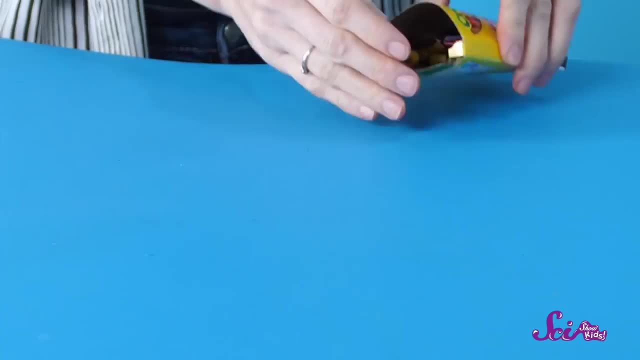 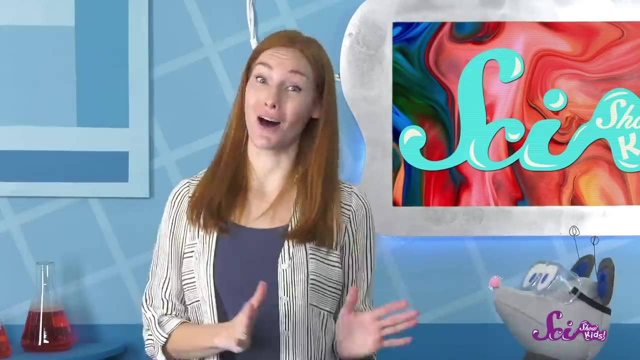 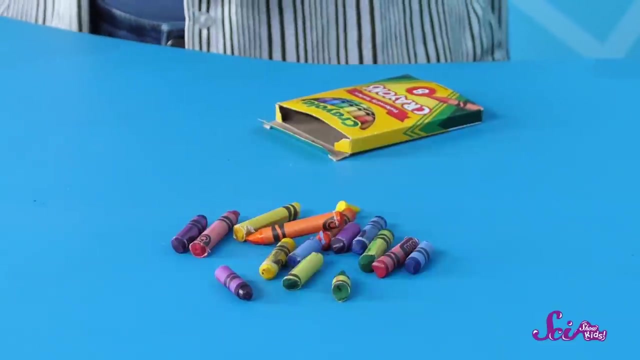 Oh, I see Squeaks is running a little low on his crayons. We've been doing a lot of coloring lately and it looks like all of his crayons are kind of worn down. It makes them a little hard to hold and really hard to use. 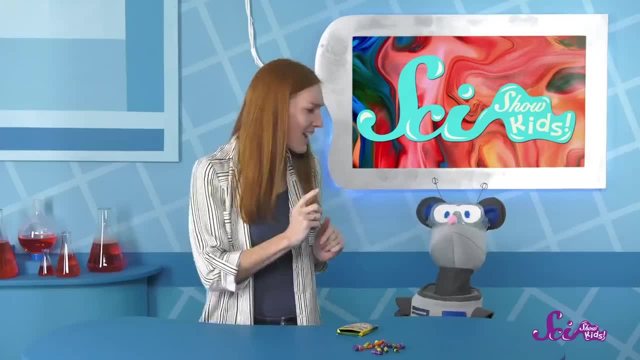 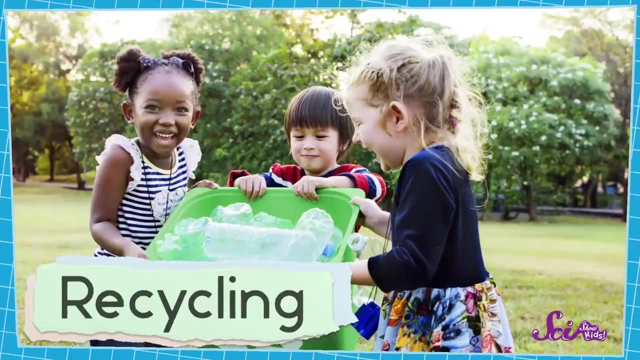 So he thinks it might be time to toss them out. Hey, I have an idea. Instead of throwing these old crayons away, why don't we recycle them? Recycling means taking something we would normally toss into the trash and turning it into something new.